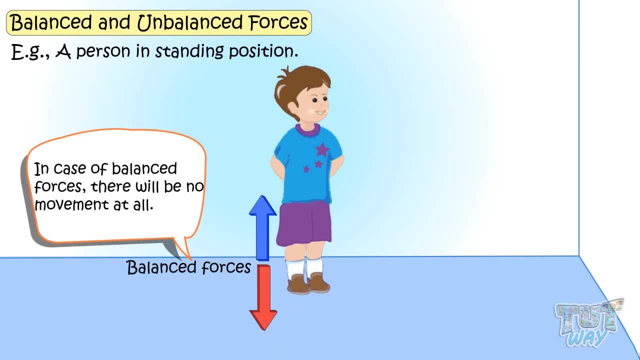 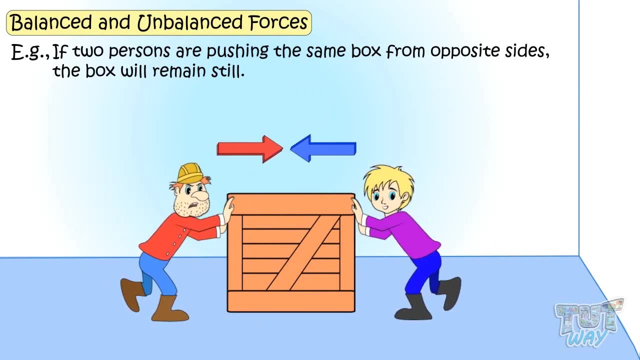 In case of balanced forces, there will be no movement at all. If there is even one force rising, I can see that there is a movement keeping on moving an object and two persons are pushing it from opposite sides- the object will stay still. 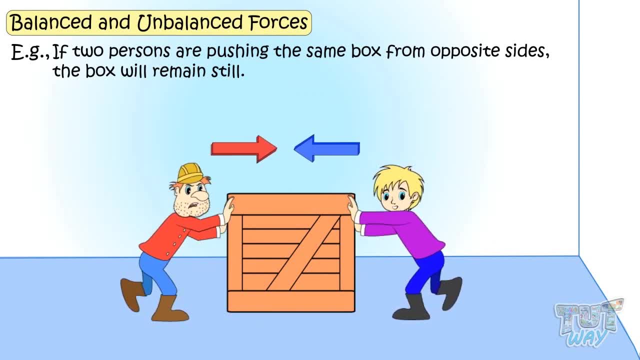 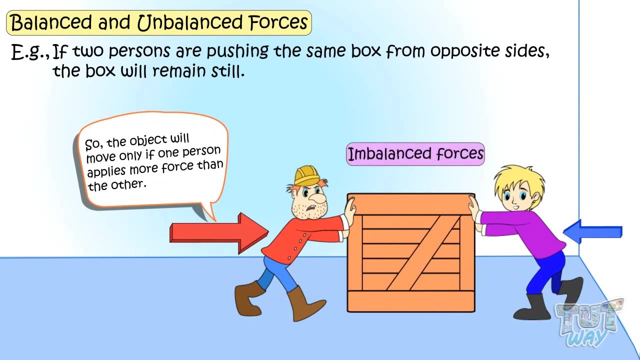 or will not move If the force acting on both the sides is the same. that is balance. forces are acting on it, So the object will move only if one of the persons applies more force than the other. That is, there is an imbalance in the forces. So movement is caused only if unbalanced. 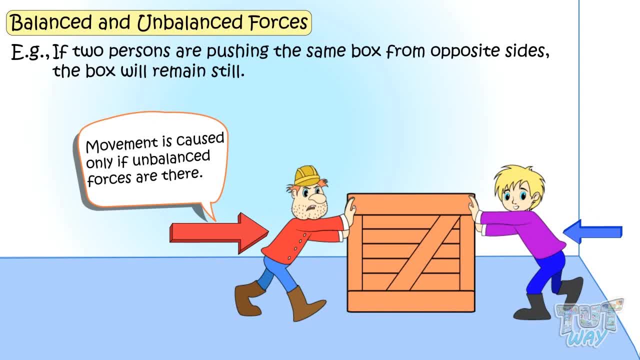 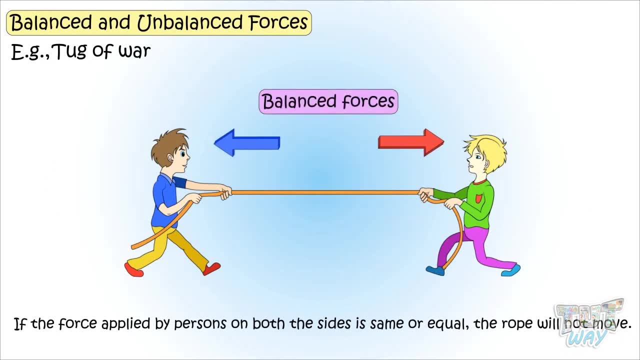 forces are there. Here is another example: in case of tug-of-war, If the force applied by persons on both sides is the same or equal, the rope will not move. The rope will move only when the force is applied more by one side of the team. 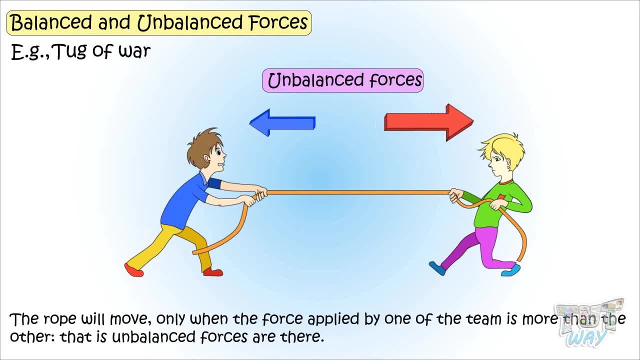 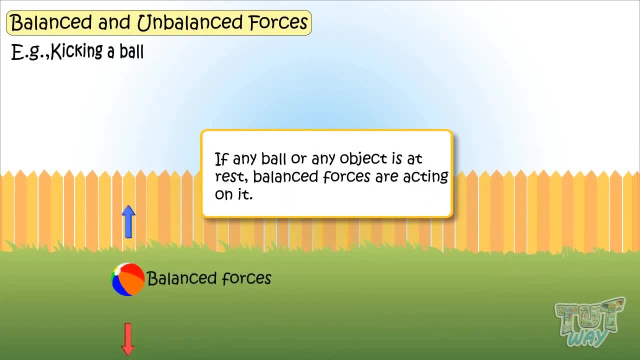 than the other other. that means unbalanced forces are there. If there is a ball at rest, it means balanced forces acting on it. Then the ball will stay at rest until some external force acts on it to shake the balance of forces acting on it. If someone kicks the ball, the force of the kick is more. 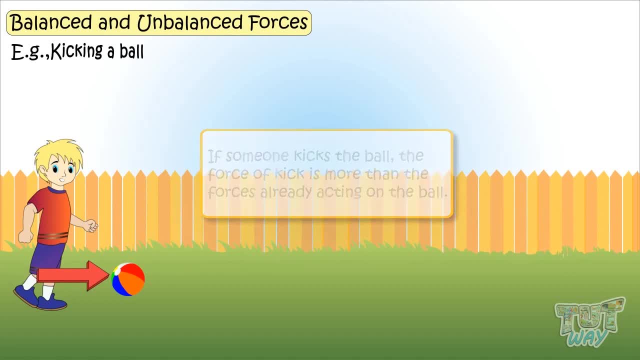 than the forces already acting on the ball. That is gravity is pulling the ball, Ground is pushing the ball. That is, both the forces were equal and opposite. That is, balanced forces were acting on the ball, but when someone kicked it, a larger force acted on the ball and there created 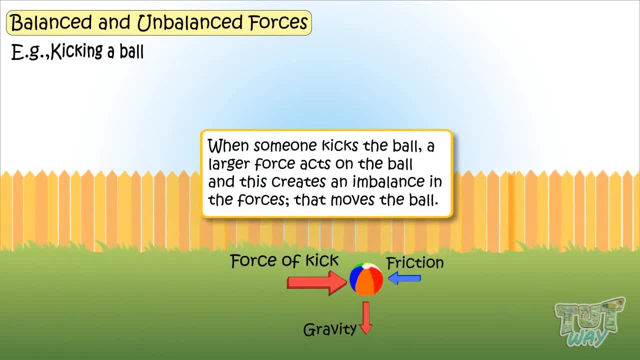 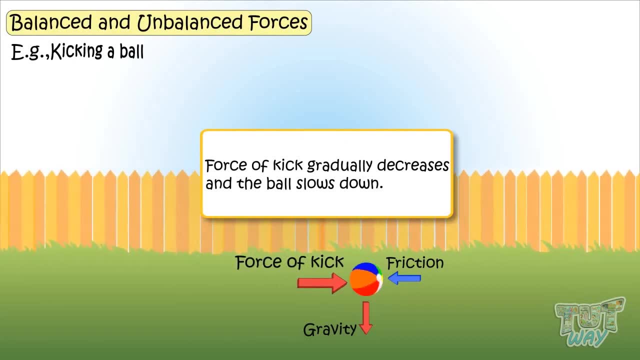 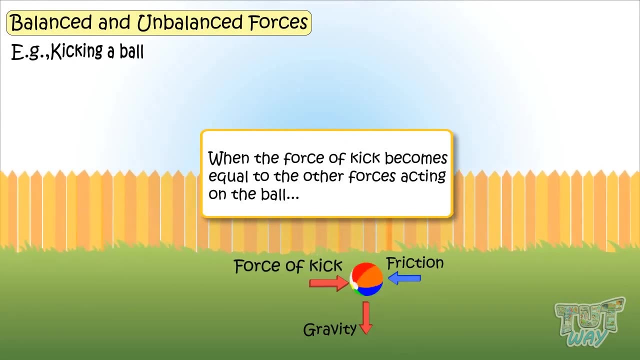 an imbalance in the forces that moves the ball. Now the force of kick gradually decreases And the ball slows down. When the force of the kick becomes equal to the other forces acting on the ball, again balanced forces are there acting on the ball and the ball stops. 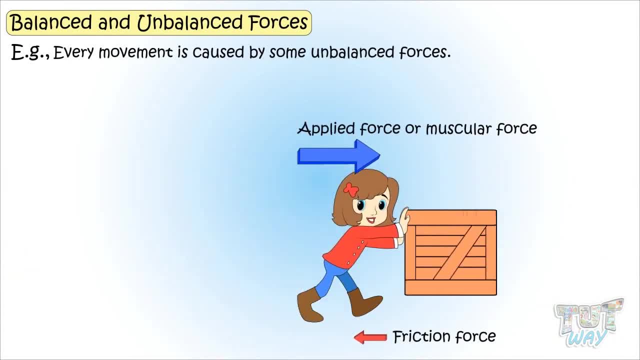 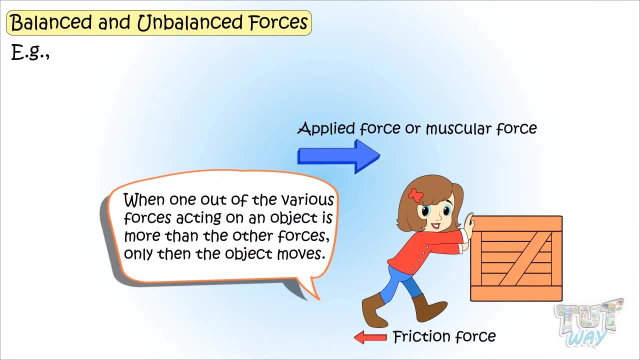 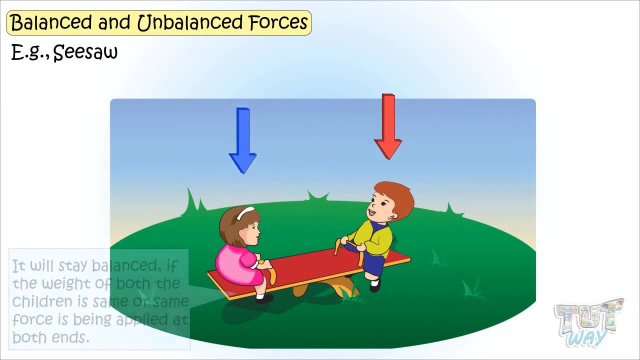 So, kids, any movement is caused by unbalanced forces. When one out of the various forces acting on an object is more than others, only then the object moves. Here is an example of a seesaw. It will stay balanced If the weight of both children is the